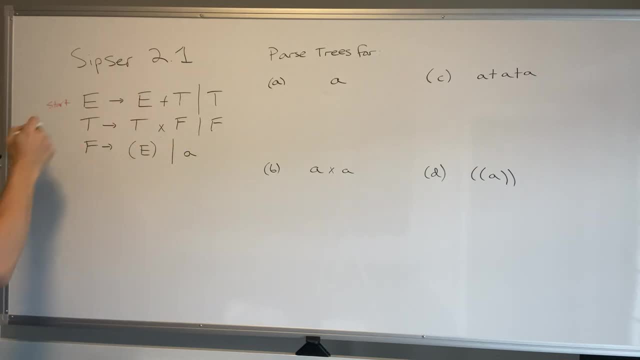 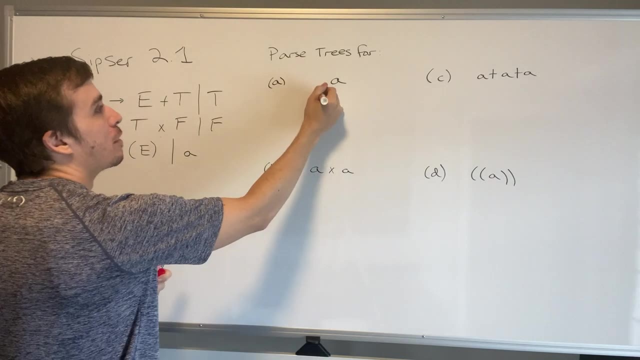 anywhere else other than right here. Okay, so we got to make a parse tree for just the letter a. now, Well, we always have to start with the start variable, so that means that we're going to make a node right here just for the start variable, which is e. 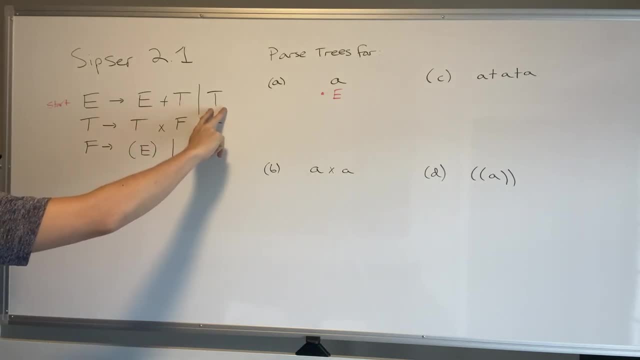 Now we have a choice of whether to apply this rule or to apply this one. Well, we can't apply this one because that means I'm going to generate the plus character and, in the contextest for grammar, you can't get rid of a terminal once you actually generate it. 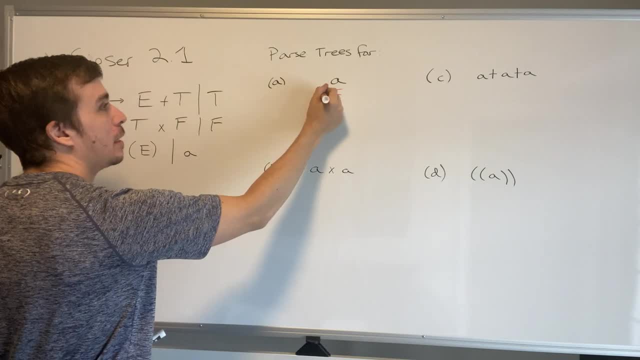 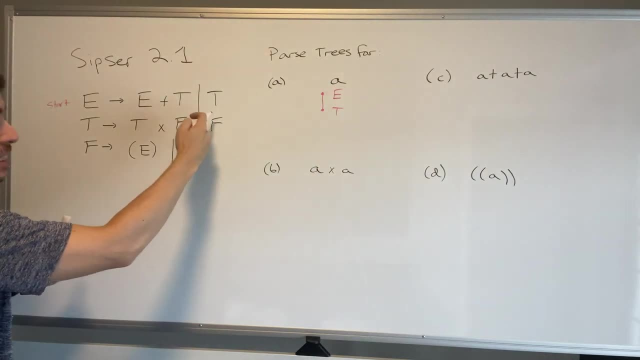 So we can't apply this one, so we got to apply that one And we're given the promise that then this grammar can actually generate the character a, at which point, if it can't, then this right hand side would fail, but we are guaranteed that it'll actually generate the thing. Okay, so now we're at t. 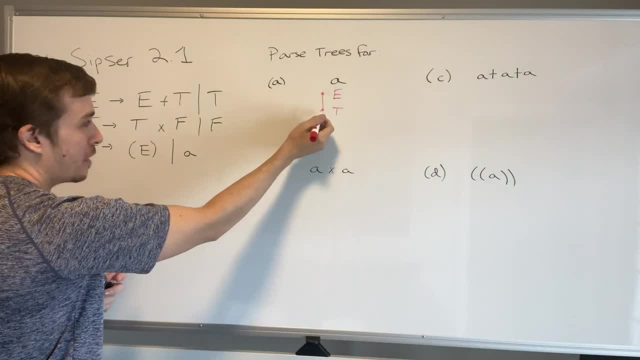 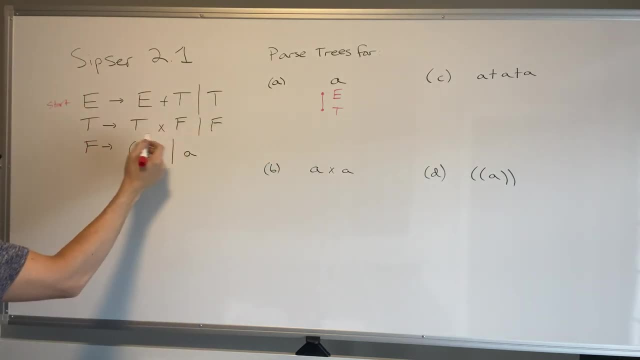 t, so the only node under here is t. so we got to work with this uh, this uh, node t. so then now t, we could apply this one again, this rule, or we can apply this one. well, we can't apply this one for the same reasons as before, because this terminal would be generated and it's not present here. 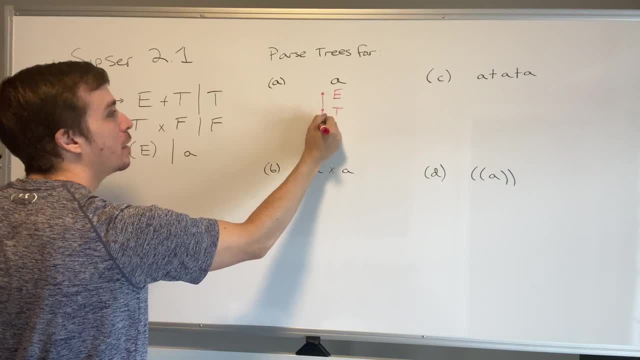 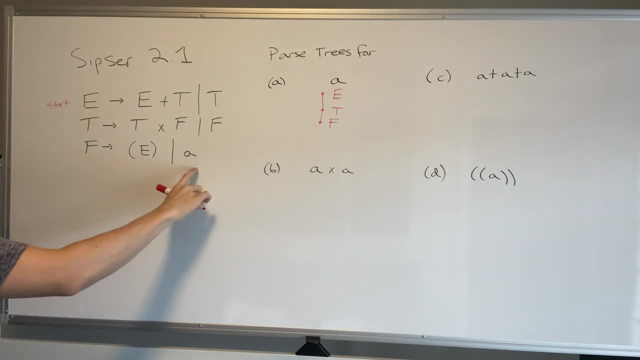 so we have to apply this one. so again, there's going to be one node under here which is going to be the f, which is the right hand side of that rule, and then now f it better be generating just that letter, that letter, a right here, because that's the. 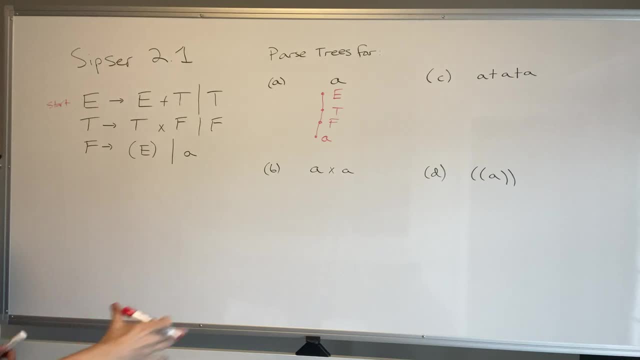 only thing in the string that we need to that we're able to generate. okay, so then now let's do this one. so again, we got to start with the start variable at the top. well then, now we can't make a plus because there's no plus here. so again, we got to go to t. then in t, well, we got the x here. 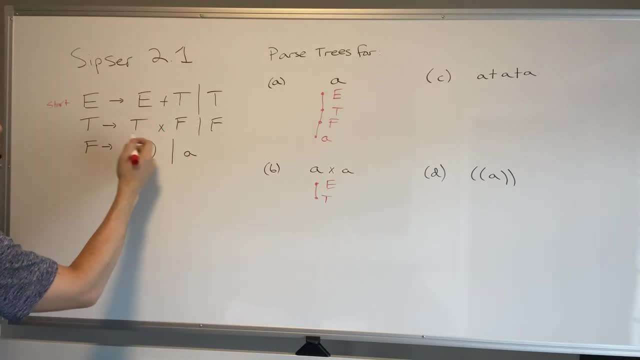 so we may or may not generate this. it turns out that we will. we'll use this rule right here instead of this one, because if we apply this one, the only way we can ever get back to the x here is if we generate the left and the right parenthesis. if we went this: 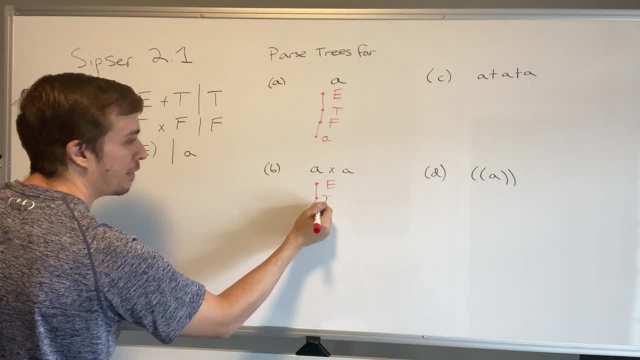 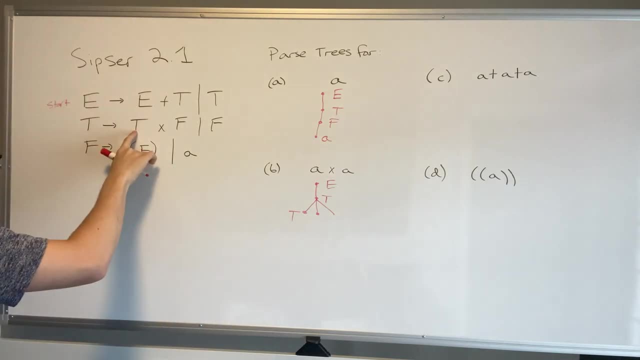 way, so we got to go this way. so then now we're going to have two children under here, which actually three, sorry. so that's going to be the t first, because that's the first thing on the right hand side, then the x, and so nothing is going to appear under the x, because it's a terminal. 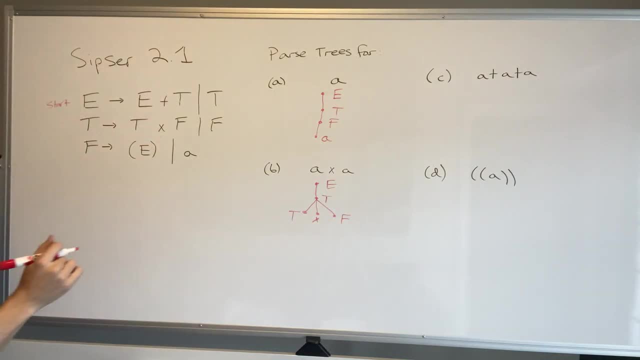 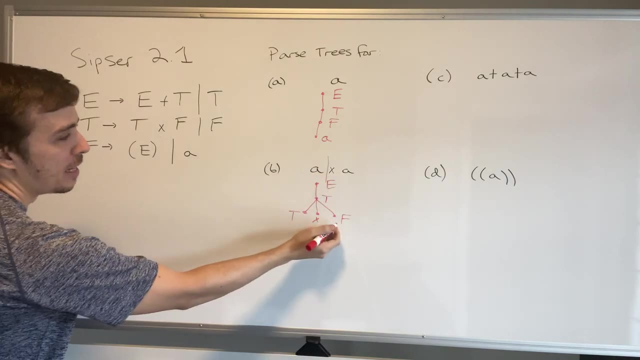 and then we have the f over here, press f in the chat. so then the t here is going to make the things that are on the left side of this x right here, and then the f is going to make the things on the right side of that x. 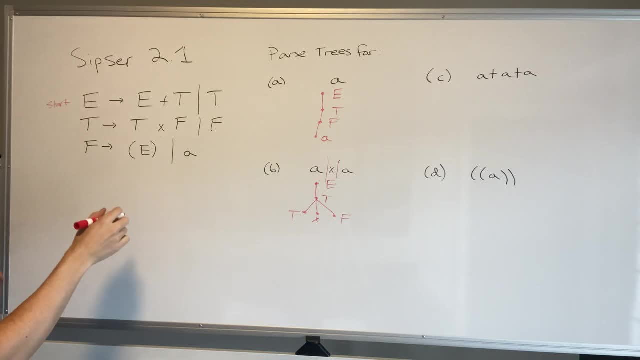 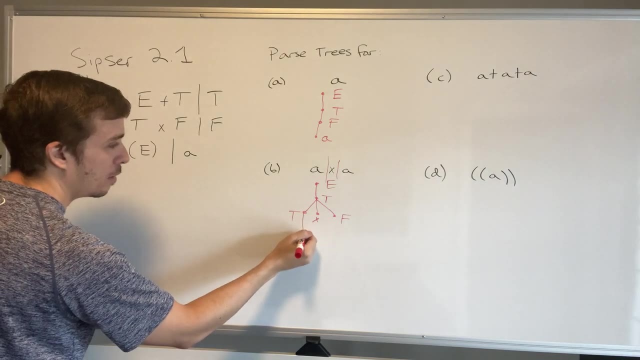 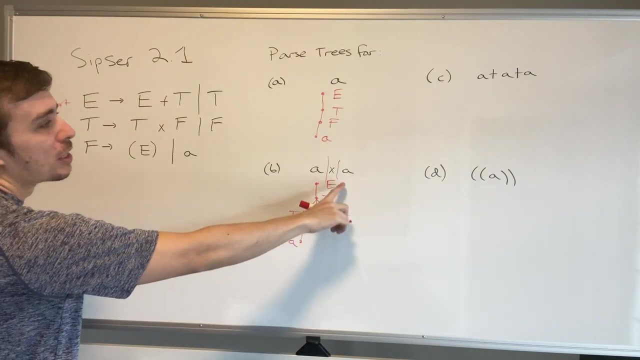 well, t is going to make just that letter a. oh, it's only responsible for that. well, t is going to get down to here, so t must do the f a route again. so we've got to go the f a route, and then the f over here is going to make the things to the right. 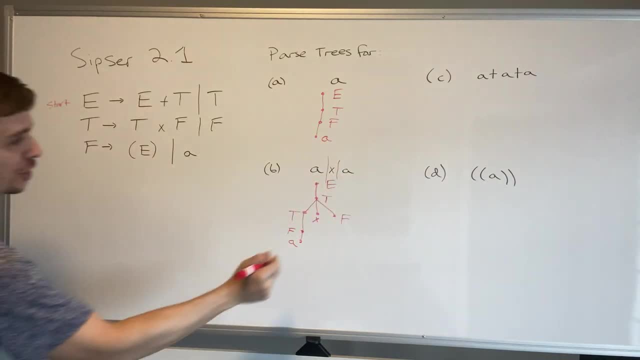 of the x, which is just an a over here, and f can just make that directly, so we can just do it pretty simply like that. all right, so then now let's do the a plus a plus a, and it's pretty clear we're gonna apply this rule twice, because there's two pluses there. 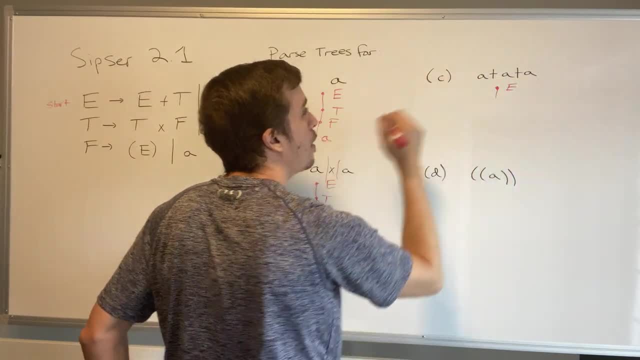 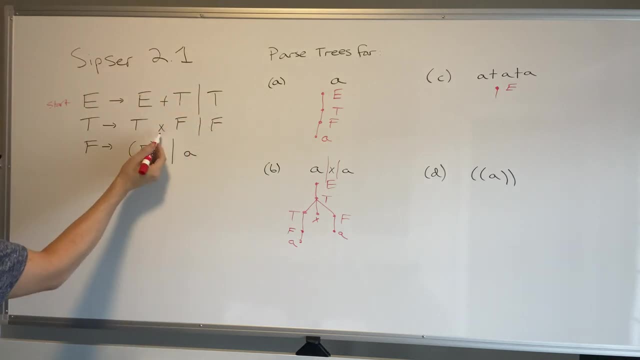 so we're gonna have e at the top, as always, and then what's underneath it? well, if we apply this one, then we could, in principle, come back up, but either we'll make the x or we're going to have preposites to be able to get back up and and execute this rule again, which we don't want to. 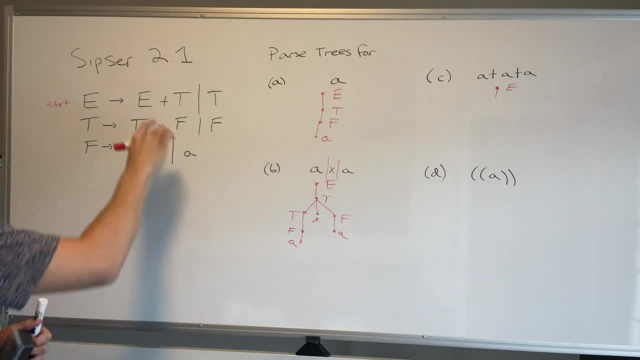 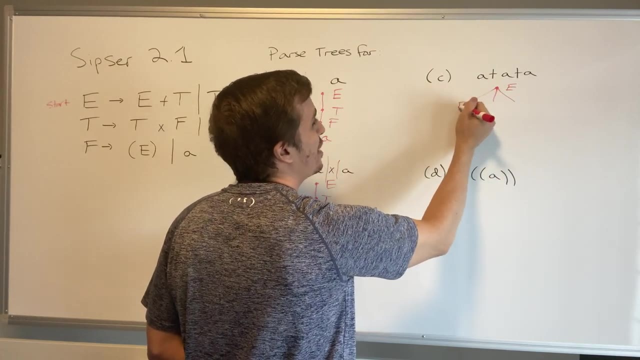 do because it's not over there. there are no parentheses over there, so now we got to apply this rule, which means that we got to have three children under here. we're prolific, we have three children, so we have an e here, then then a plus, and there's going to be no. 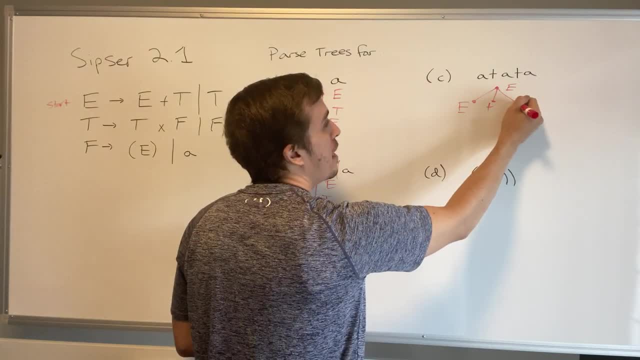 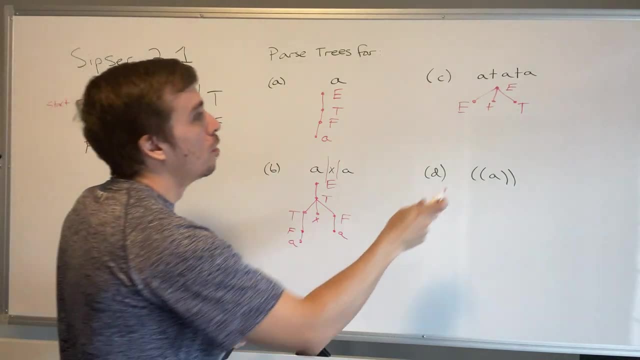 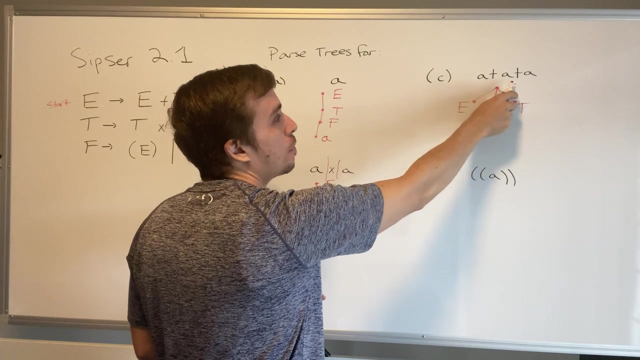 children under this, because that is a terminal, and then we're going to have, in this case, a t, then that means that we have a choice. now, well, it turns out we won't have a choice, but in principle we have a choice. what does this plus refer to? does it mean the left plus or the right plus? 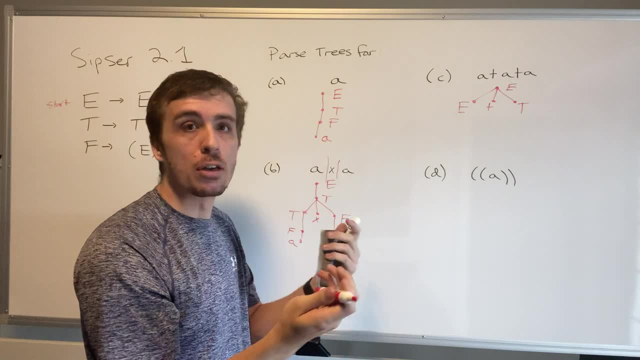 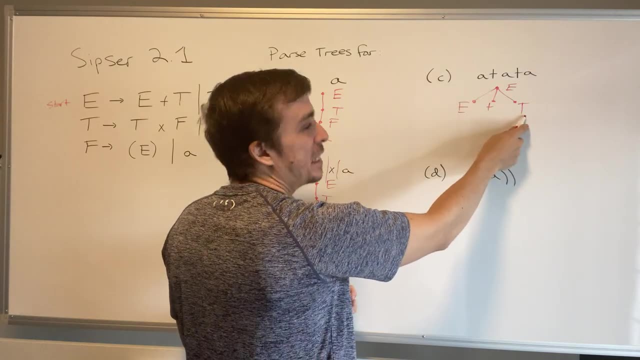 well, in principle it could be either, because it's a context-free grammar. it turns out that it'll be the right plus, and the reasoning is that if this was the left plus, then the t right here has got to make the right plus. well, in order for t to make the plus, it's got to. 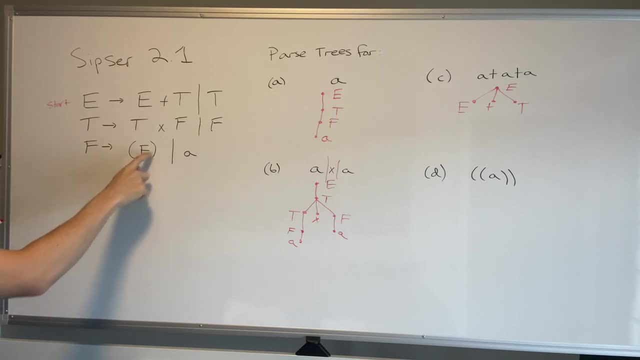 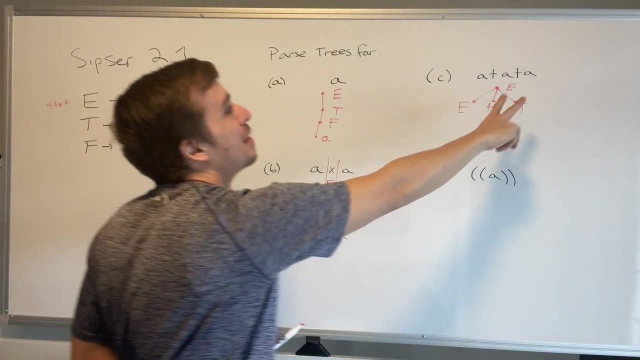 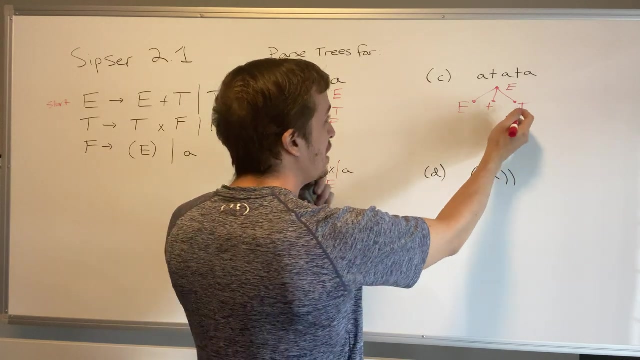 do the f-rule. it's going to go through the f-rule and then come back up to be able to get the other plus. well, here, then that means it's got to make parentheses, and there's no parentheses on the right hand side over here, so that means that this plus must be this one, and so therefore, 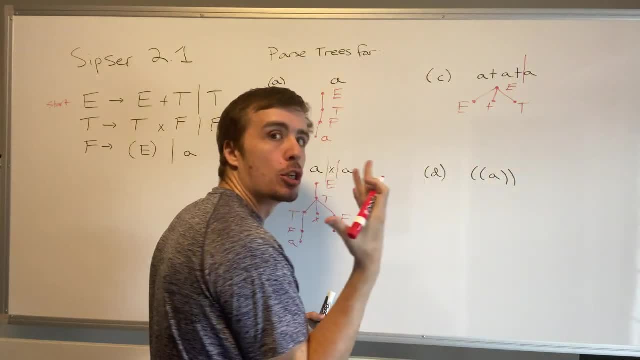 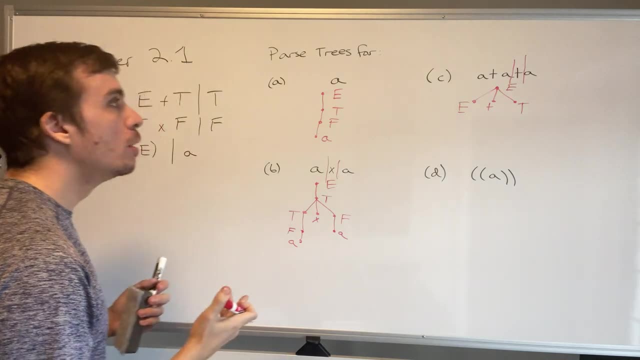 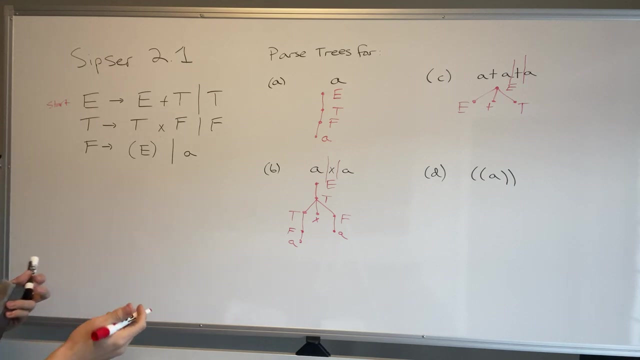 this t right here is going to be responsible for everything to the right of that plus, and then the e here is going to be responsible for the things to the left of it. so this kind of grammar is called well, it's a context-free grammar, but the e kind of is like an expression in some sense. 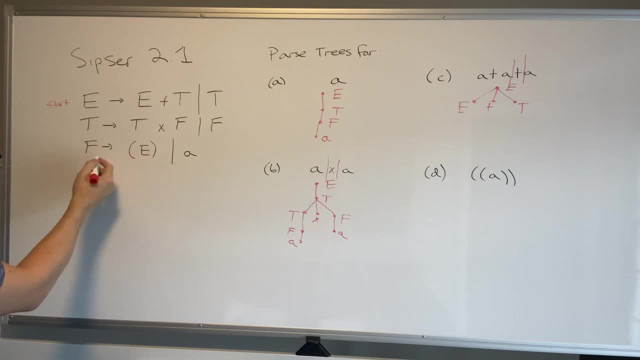 You can add two expressions or multiply two expressions, or you have an expression within parentheses or a character, And so this is used in programming, language parsing, But anyway, so here this e is going to make this stuff well. it can do the plus directly. So this e is going. 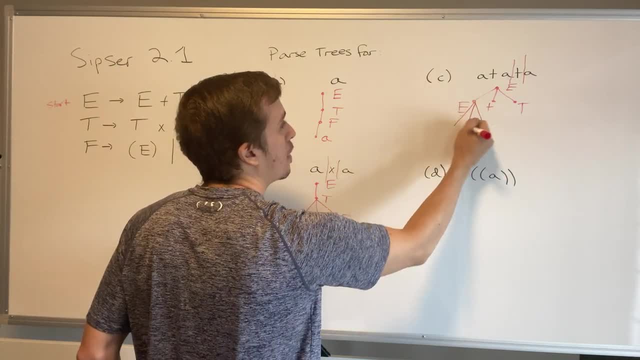 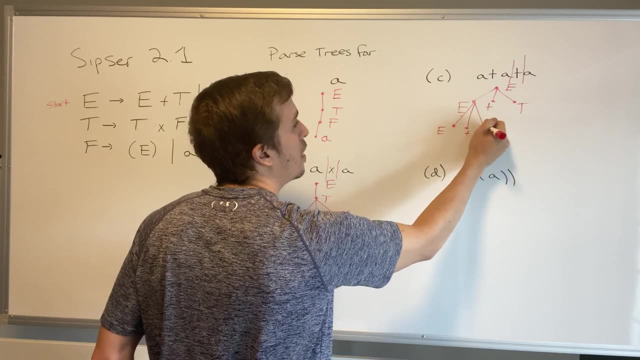 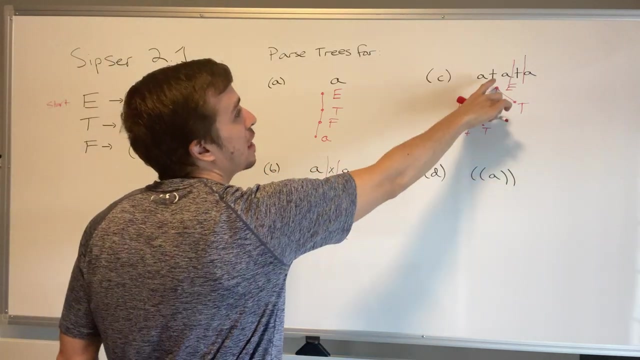 to have itself have three children. So it's going to have an e on the left side, a plus, not a plus, and then a t here. So nothing under this plus again, because it's a terminal. Well, this plus is the left one, so this e has to make the singular a right here. So again we got. 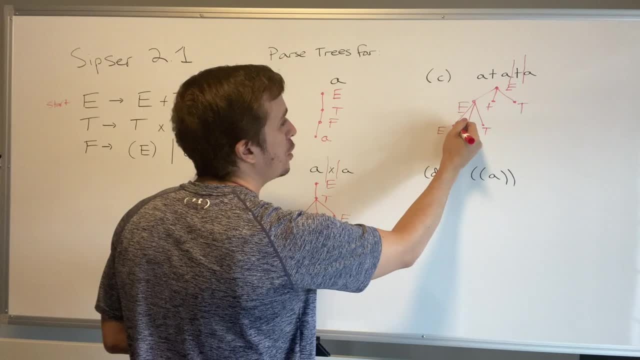 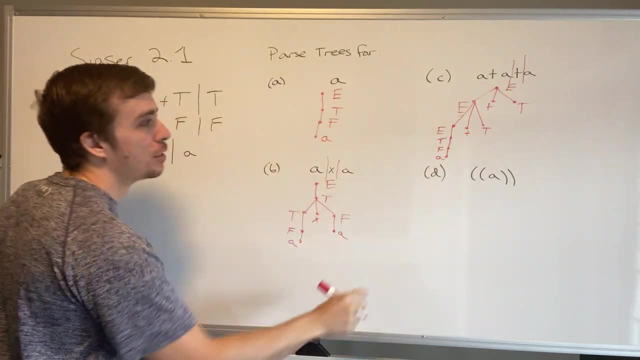 to go through the grammar from e all the way through. So this e is going to make a t, which is going to make an n. This f needed to give myself more room here, probably, So it's going to make the e, it's going. 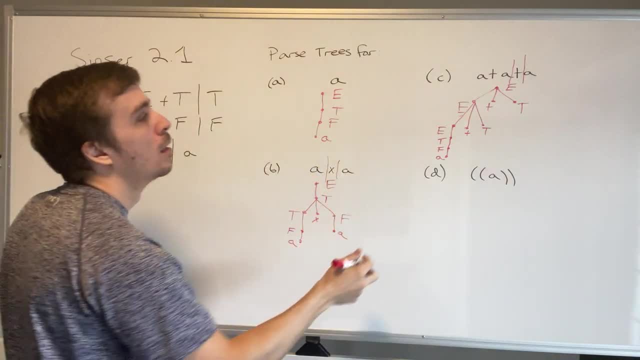 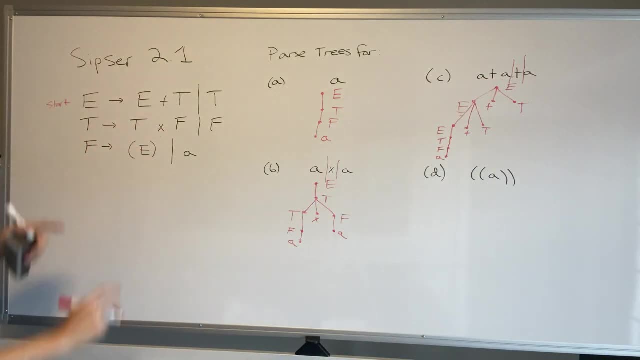 to make the t, make the f, make the a, just like we did before. Well, this t is going to make that middle a, and we can pretty easily do that just by doing t, f, a. So t is going to make f, which is: 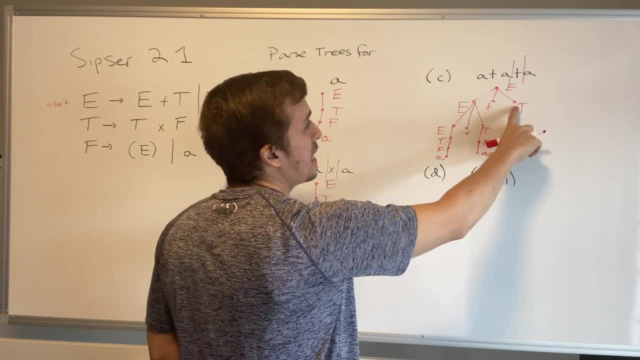 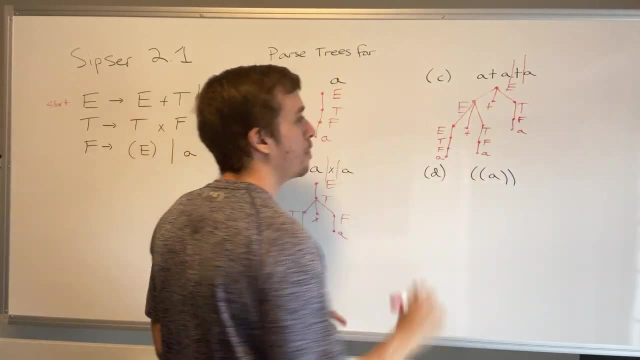 going to make a, All right, then this t is going to make that final a, and so we just did that work. So t f a like that. And this is a unique parse tree because of the reasoning we had, that this plus had to. 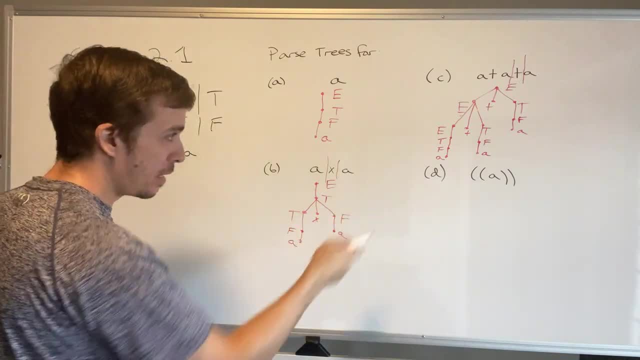 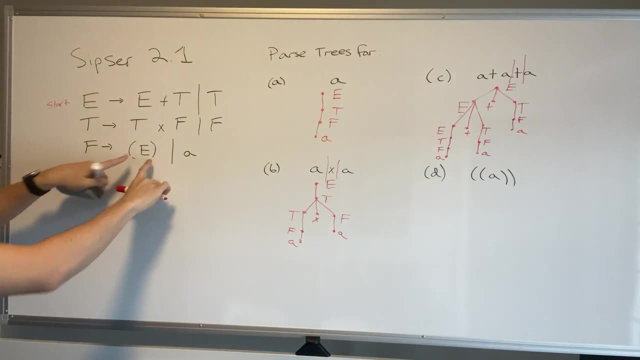 mean the right one and not the left one. All right, so then now let's do this guy which has double nested parentheses. So that means, effectively, we've got to apply this rule twice, but that means that since there's an e inside here, that means we got to go all the way.